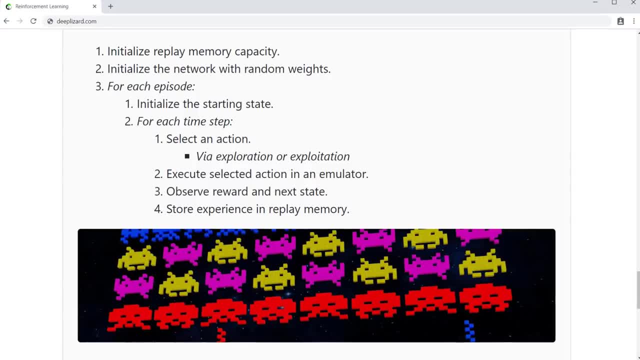 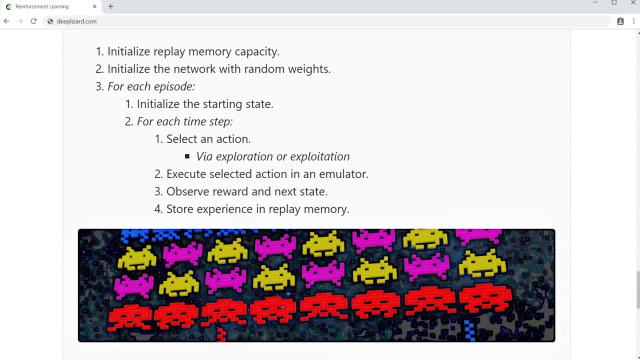 replay memory. As a reminder, here's a snapshot summary of what all we covered before we ended last time. Make sure you've got an understanding of all this. All of these steps have occurred before the actual training of the neural network even starts. 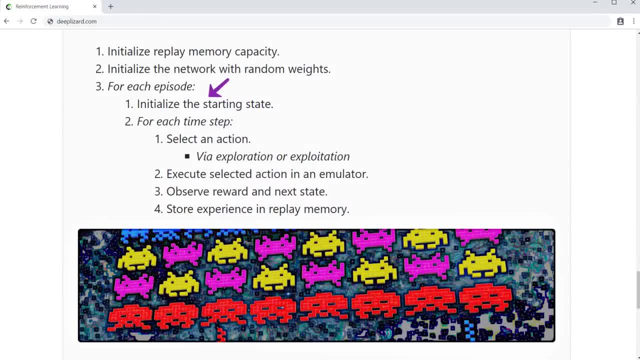 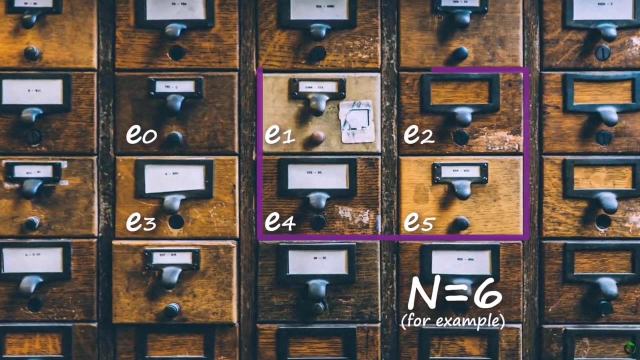 So at this point we're inside of a single time step within a single episode. Now we'll pick up right where we left off, after the experience tuple is stored in replay memory to discuss what exactly happens during training. After storing an experience in replay memory, we then sample a random batch of experiences. 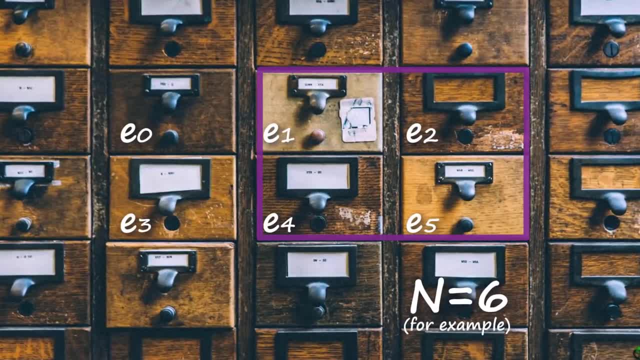 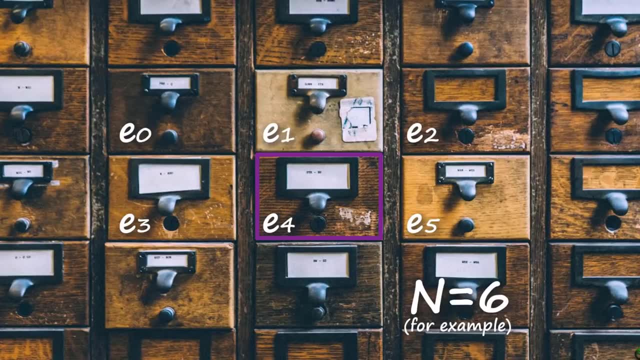 from replay memory. For ease of understanding, though, We're going to explain the remaining process for a single sample rather than for a batch, And then you can generalize this idea to an entire batch. Alright, so from a single experience sample from replay memory, we then preprocess the. 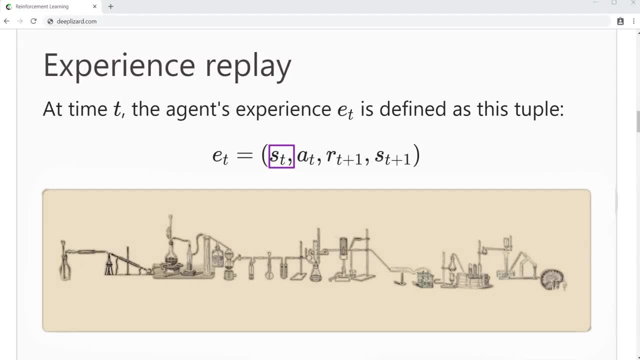 state by doing normal grayscale conversion, cropping, scaling, etc. And we then pass the preprocessed state to the network as input. In reality, though, remember we discussed that a single state will likely be made up of a stack of frames, for example. 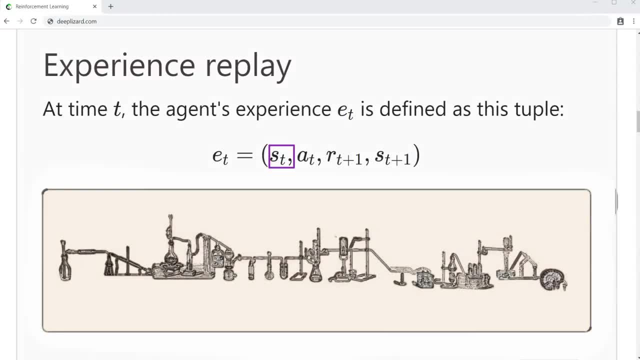 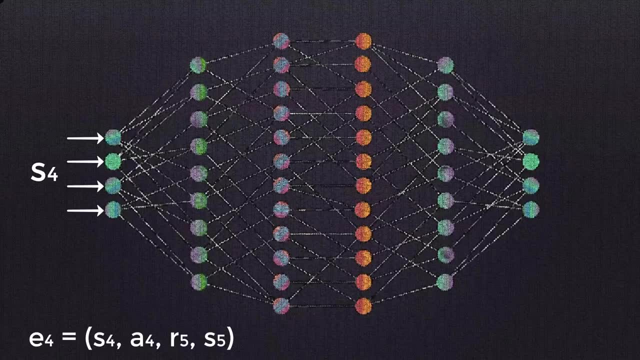 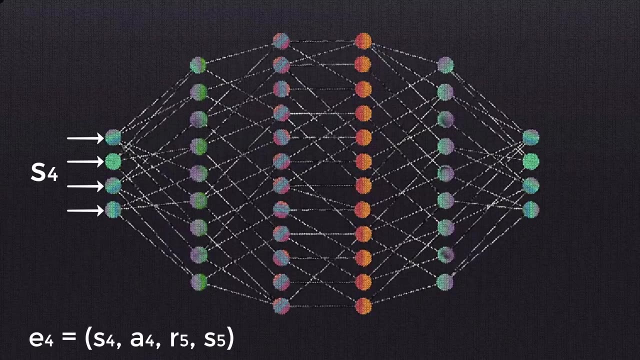 So that we can have context in regards to movement in the environment. Going forward, we'll refer to this network as the policy network, since its objective is to approximate the optimal policy by finding the optimal Q function. The input state data then forward, propagates through the network with the same forward. 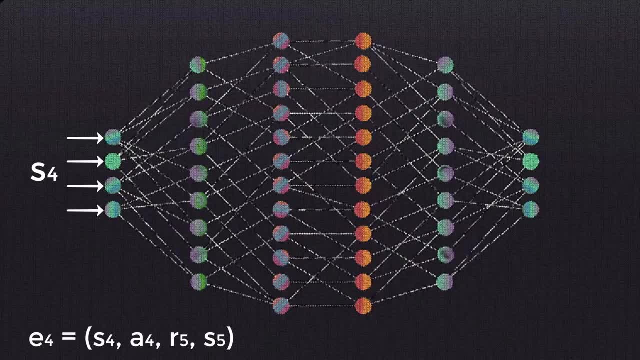 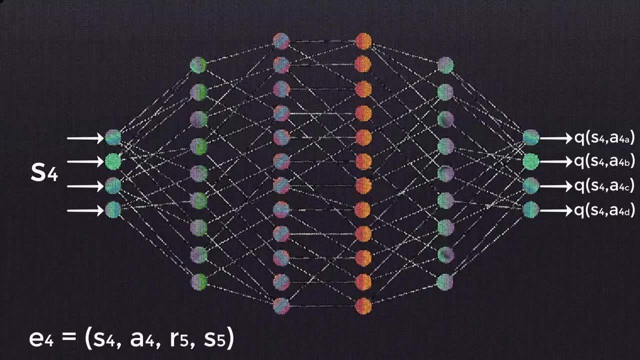 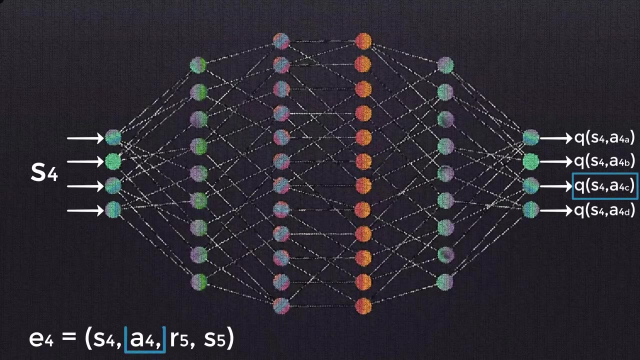 propagation technique that we've discussed for any other general neural network. The model then outputs an estimated Q value for each possible action from the given input state. At this point the loss is there. It's then calculated. We do this by comparing the Q value output from the network for the action in the experience. 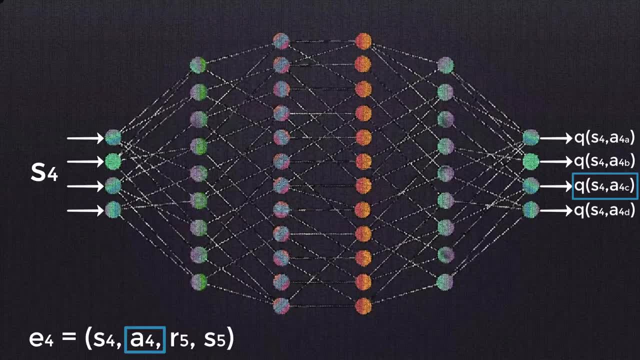 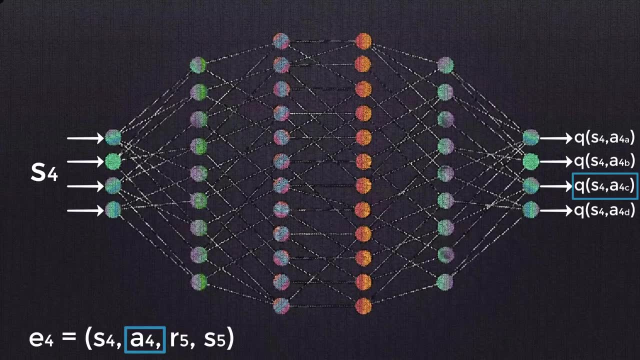 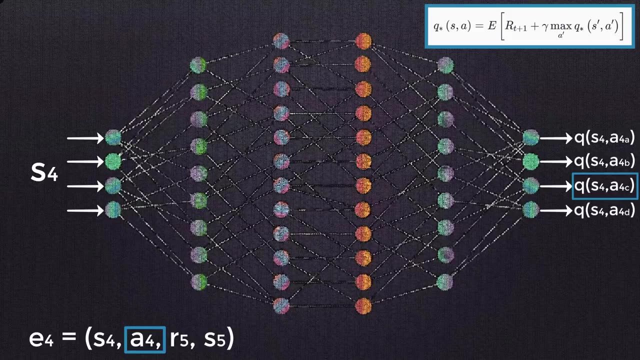 tuple we sampled and the corresponding optimal Q value or target Q value for the same action. Remember, the target Q value is calculated using the expression from the right-hand side of the Bellman equation. So, just as we saw when we initially learned about plain Q learning earlier in this series, 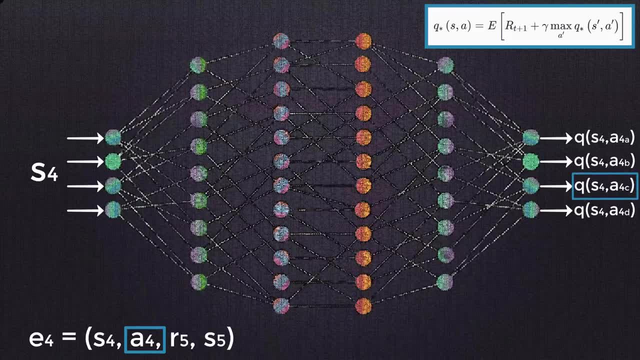 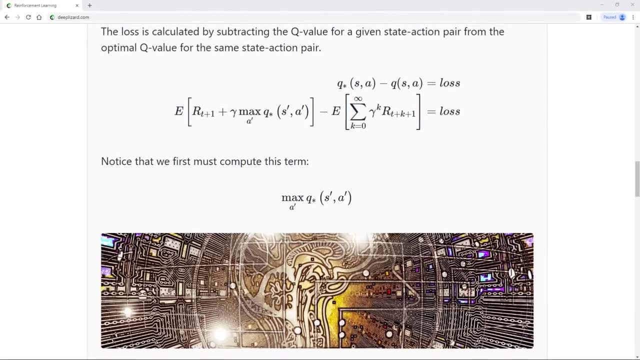 the loss is calculated like this: We subtract the Q value for a given state action. Now, when we're calculating the optimal Q value for any given state action, pair, notice from the equation for calculating loss that we have this term here, that we must compute. 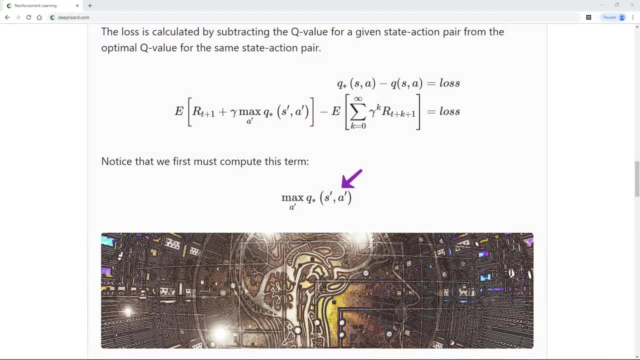 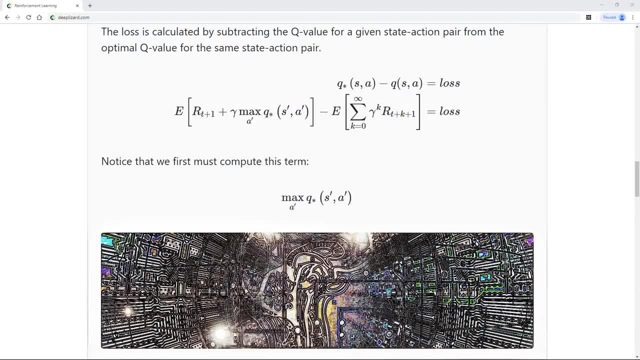 We'd just look to see which action gave us the highest Q value for a given state action. Well, that's old news. now, with deep Q learning, In order to find this max term now, what we do is pass S' to the policy network, which 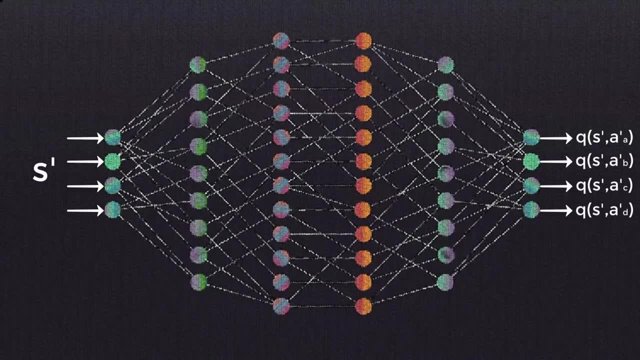 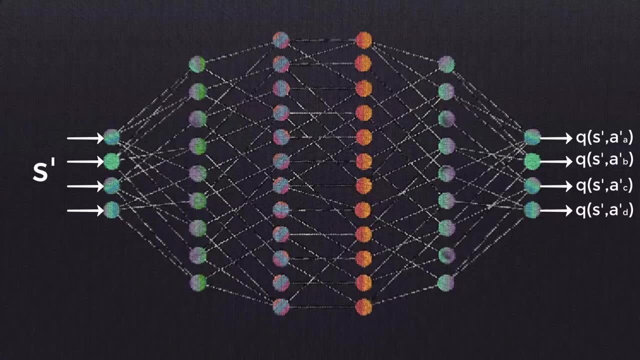 will output the Q values for each state action pair using S' as the state and each of the possible next actions as A'. Given this, we can obtain the max Q value over all possible actions taken from S' giving us this max term that we're after. Note that, for our specific example, we're going to use S' as the next action. Note that, for our specific example, we're going to use S' as the next action. Note that, for our specific example, we're going to use S' as the next action. 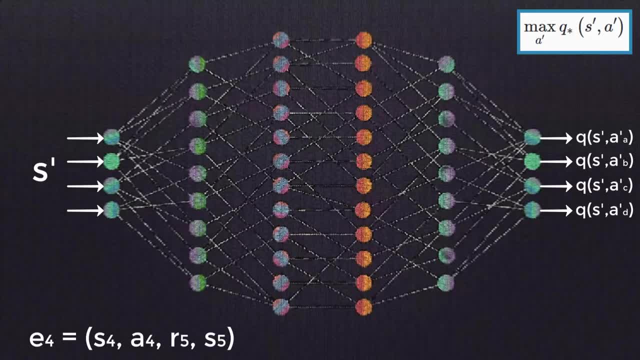 For our specific example, we're working with Experience Tuple E4, so our initial state we passed to the network was S4. The general S' and A' notation then would take on S5 and A5 as the next state and action. 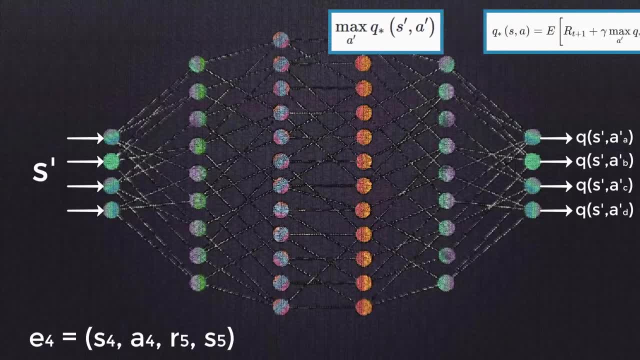 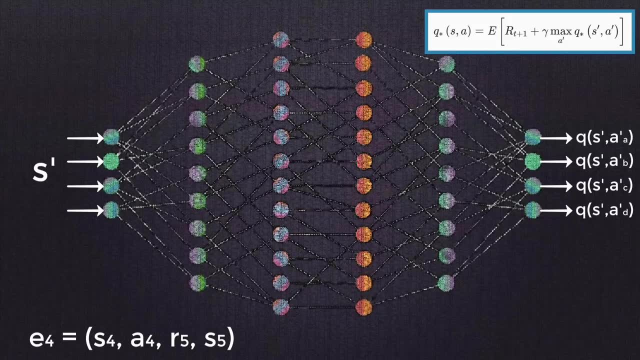 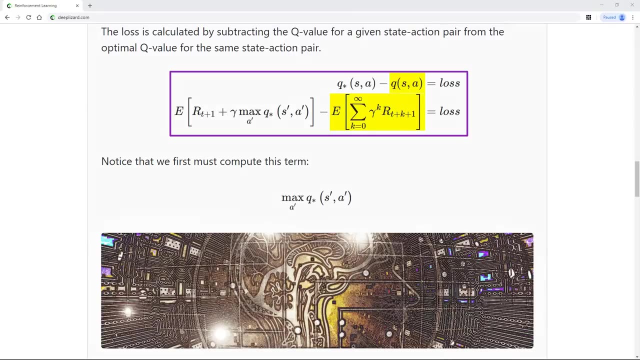 Once we find the value of this max term, we can then plug it in to calculate this term for the original State input passed to the policy network. Why do we need to calculate this term again? Ah yes, This term enables us to compute the loss between the Q value given by the policy network for 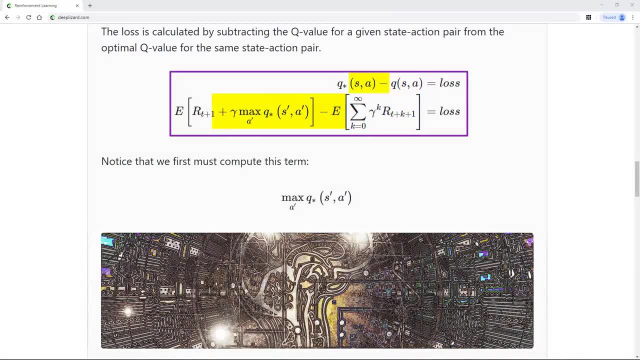 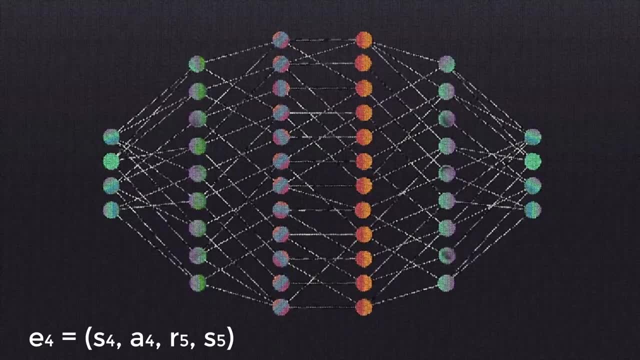 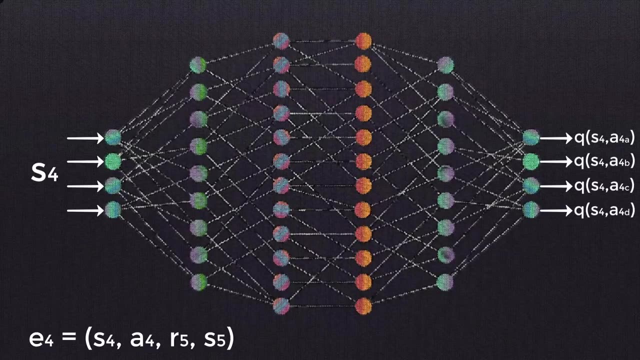 the state action pair from our original experience tuple and the target optimal Q value for this same state action pair. So to quickly touch base, note that we first forward passed the state from our original experience tuple to the network and got the Q value for the action from our experience. 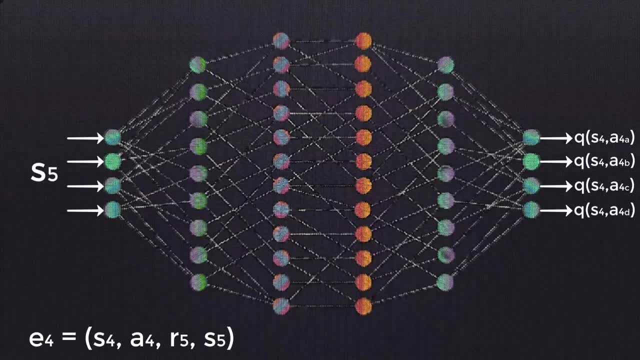 tuple as output. We then passed the next state contained in our experience tuple to the network to find the max Q value among the next actions that can be taken from that state. This second step was just done to aid us in calculating the loss for our original state. 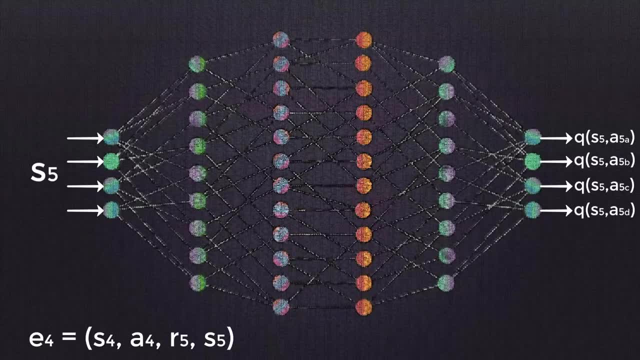 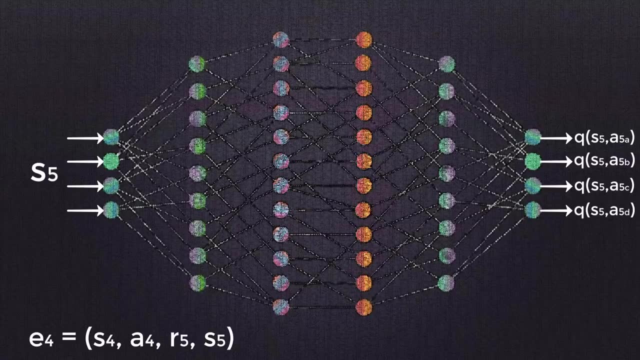 action pair. This may seem a bit odd, doing two forward passes before we even do any type of gradient update, but let it sink in for a minute and see if the idea clicks. Alright. so after we're able to calculate the optimal Q value for our state action pair. 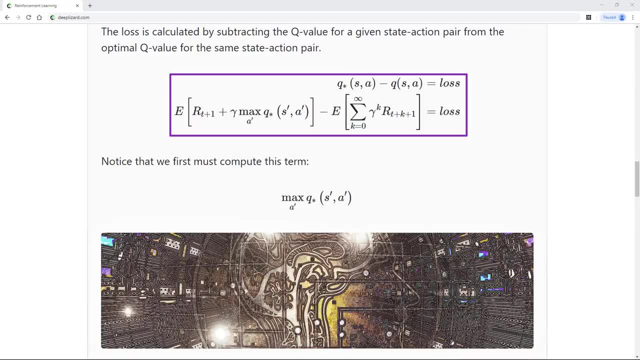 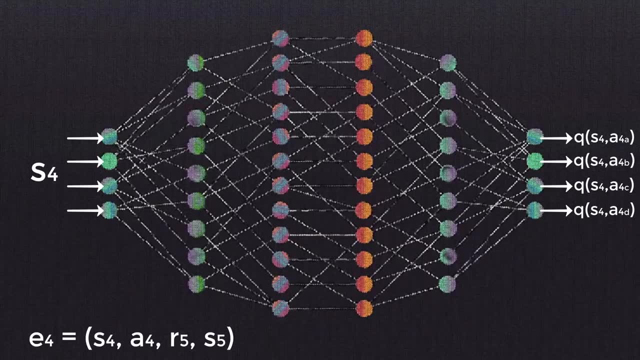 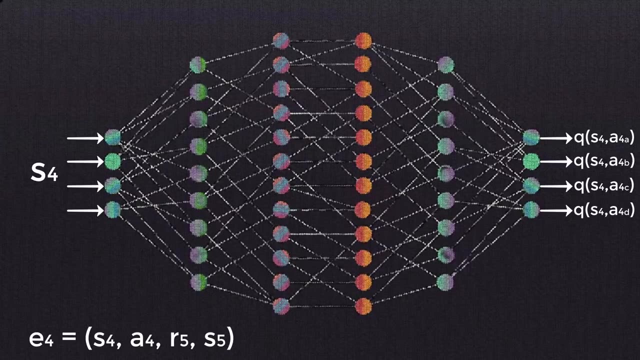 we can then calculate the loss from our policy network between the optimal Q value and the Q value that was output from the network for this state action. pair Gradient descent is then performed to update the weights in the network in attempts to minimize the loss, just like we've seen in all other previous networks that we've covered. 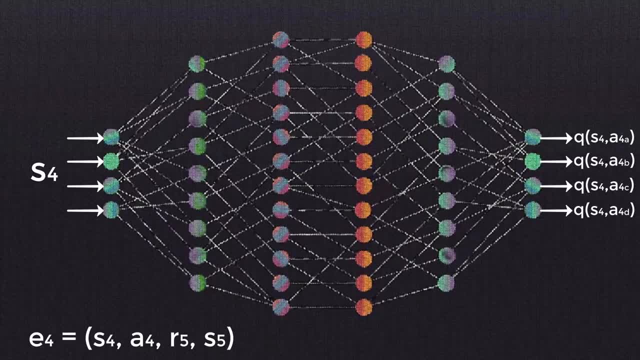 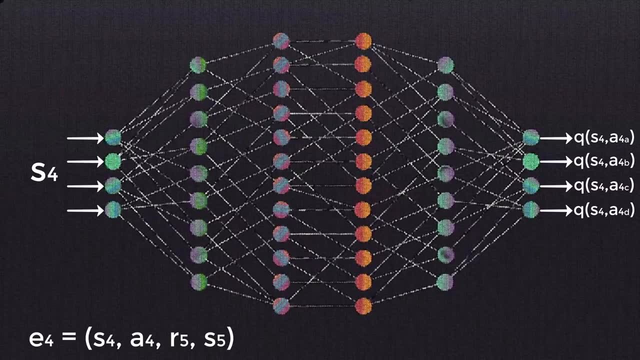 on this channel. In this case, minimizing the loss means that we're aiming to make the policy network output Q values for each state action pair that approximate the target Q values given by the Bellman equation. This will ultimately approximate the optimal Q function for each state action pair and 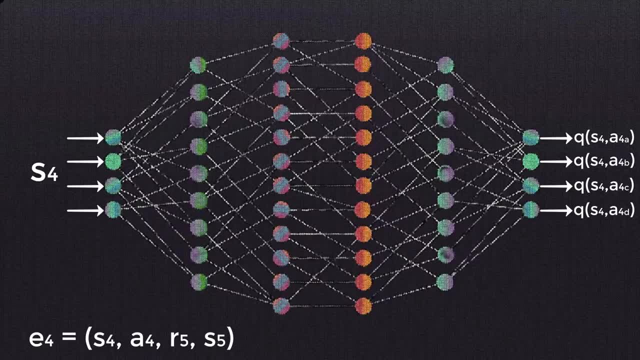 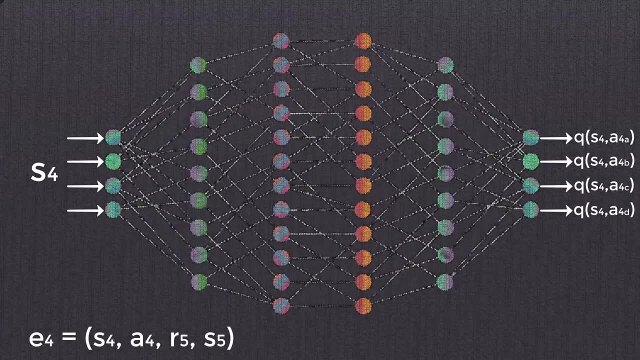 we can then calculate the target Q values given by the Bellman equation. Up to this point, everything we've gone over was all for a single time step. We then move on to the next time step in the episode and do this process again and again. 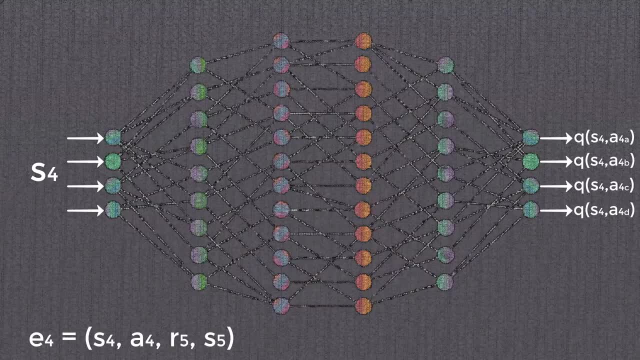 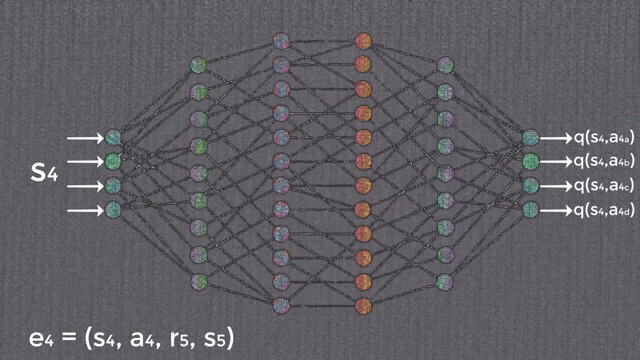 time after time until we reach the end of the episode. At that point we start a new episode and do that over and over again until we reach the max number of episodes we've set. We'll want to keep repeating this process until we've sufficiently minimized the loss. 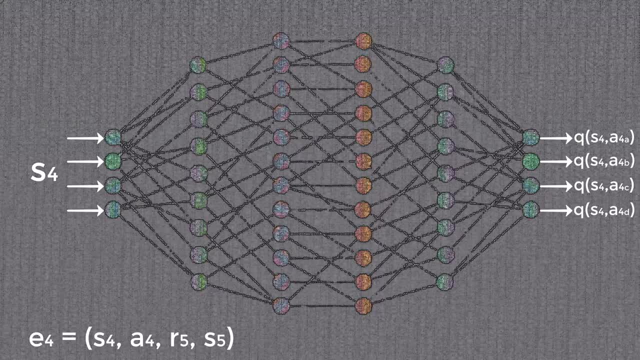 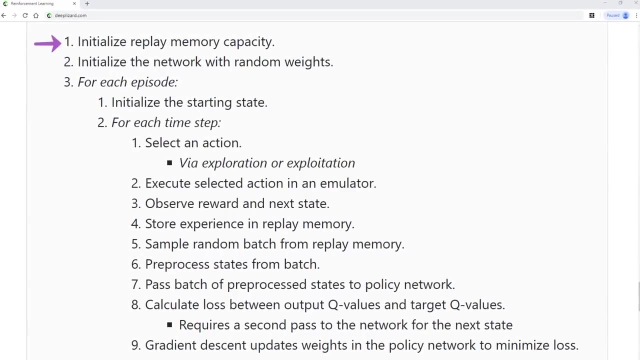 Admittingly, between the last two episodes we've only reached the maximum number of episodes, So let's go over this quick summary. to bring it all together, We first start out by initializing the replay memory capacity. We then initialize the network with random weights. 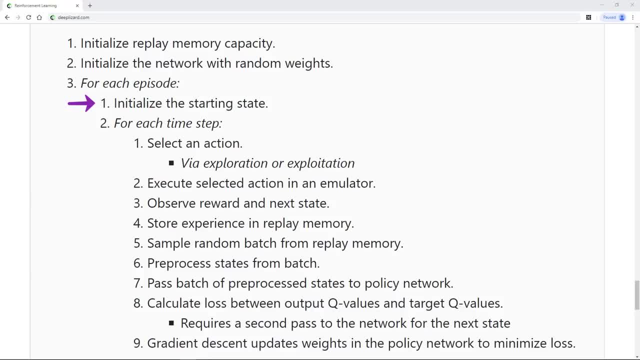 For each episode. we then initialize the starting state. For each time step within the episode, we select an action via exploration or exploitation. We then execute that selected action in an emulator, Observe the action, Observe the reward and next state and store the entire experience, tuple in replay memory.